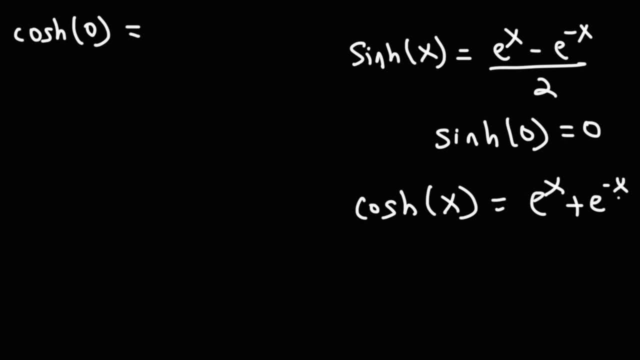 It's e to the x plus e to the negative x divided by 2.. So this is going to be e to the 0 plus e to the negative x divided by 2.. So we're going to need to know the formula for hyperbolic cosine of 0.. 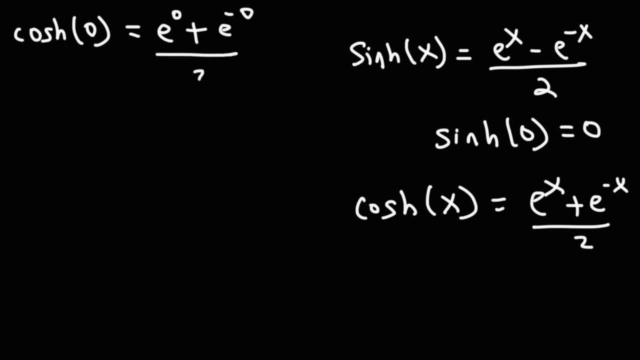 So this is going to be e to the 0 minus e to the negative: x divided by 2.. plus e to the negative: 0 over 2.. e to the 0 is 1.. e to the negative: 0 is the same as. 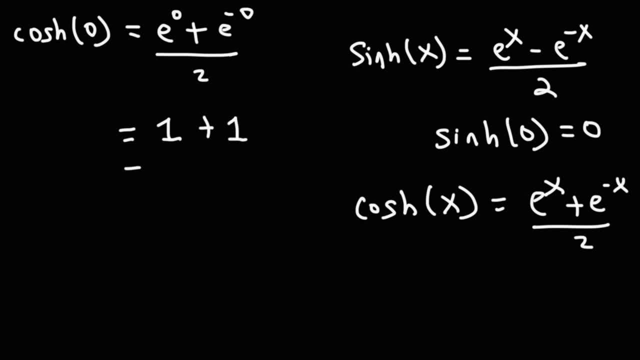 e to the 0, which is going to be 1.. 1 plus 1 is 2.. 2 divided by 2 is 1.. So hyperbolic cosine of 0 is equal to 1.. Much in the same way that sine 0 is. 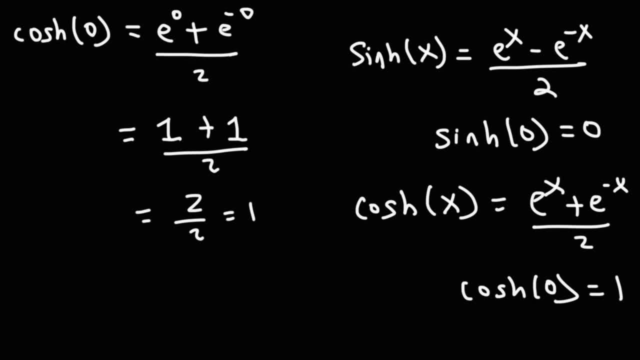 equal to 0 and cosine 0 is 1.. Try this one. What is the value of hyperbolic sine of ln 2?? Go ahead and work on that problem. So this is going to be e raised to the ln 2. 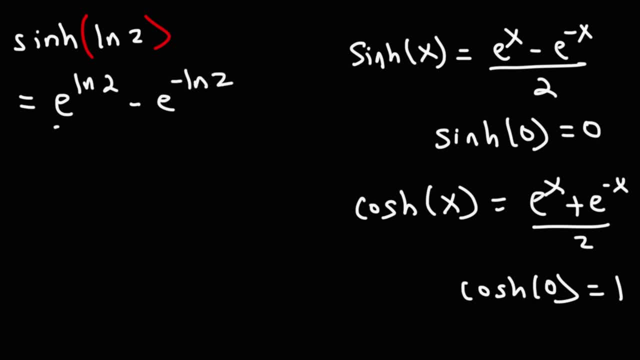 minus e to the negative ln2 over 2.. Now what is e to the ln2?? When dealing with natural logs, you have a base e. here It turns out that these cancel out and you just get 2.. For the next one, this negative 1, I want to move it to the exponent of 2.. 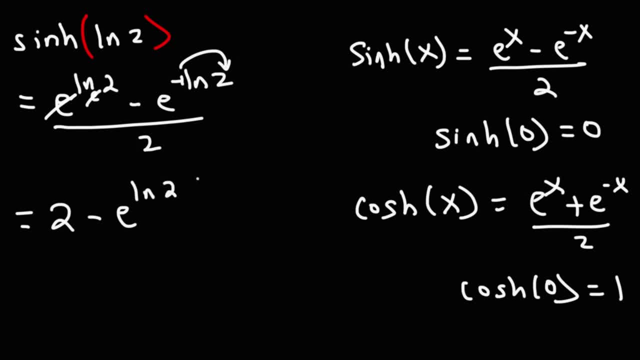 That's a property of logs that will allow me to do so. So this will be ln2 to the minus 1.. 2 to the negative 1 is the same as 1 half, So these will cancel and I'm just going to get 1 half here. 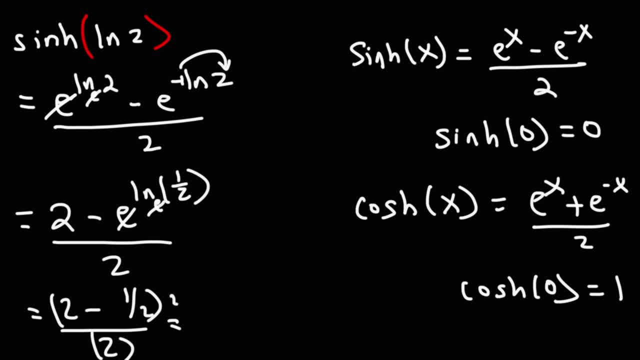 Now what I'm going to do is I'm going to multiply the top and bottom by 2, just to get rid of the fraction. So here I have 2 times 2,, which is 4.. 2 times 1, half is 1.. 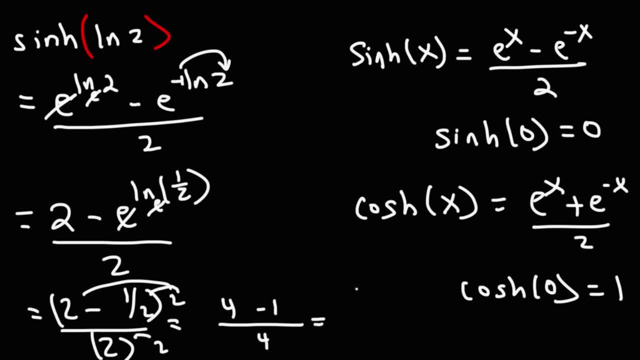 And on the bottom, 2 times 2 is 4.. 4 minus 1 is 3, so I get 3 over 4 as the final answer. So that's the value of hyperbolic sine of ln2.. It's 3 over 4.. 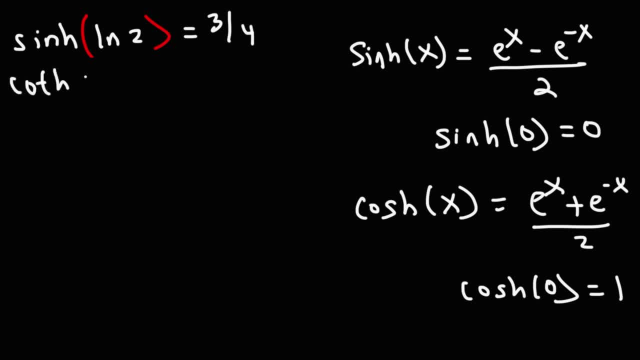 Try this one. What is the value of, What is the value of hyperbolic cotangent of ln5?? So hyperbolic cotangent- I'm going to put it here- is hyperbolic cosine over hyperbolic sine. Here we have cosine. 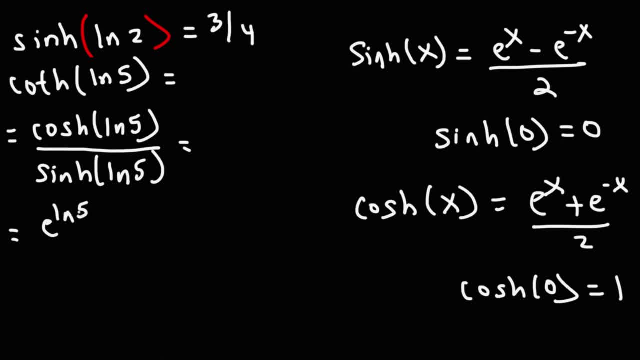 So this is going to be e to the ln5 plus e to the negative ln5 divided by 2.. And then for hyperbolic sine of ln5, we're going to use this formula. So it's e to the ln5 minus e to the negative ln5 over 2.. 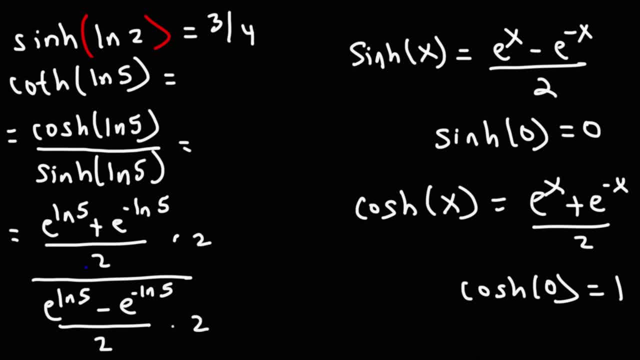 So, multiplying the top and bottom by 2, we can get rid of this. So this is going to be e to the ln5 plus, e to the ln5 minus, e to the negative ln5 over 2.. Now e to the ln5 is simply 5.. 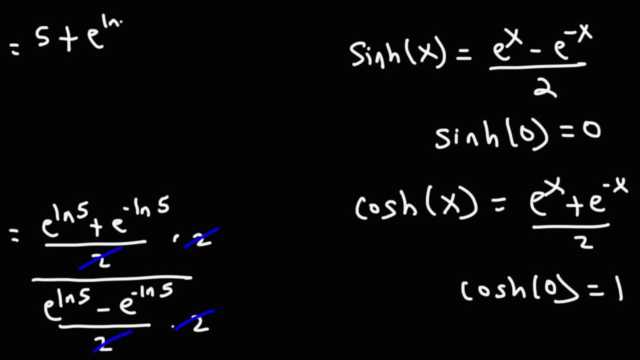 And this is going to be plus, e to the ln5 to the minus 1, or 1 over 5, over 5, minus, And we could do the same thing here. This is going to be e to the ln, 1 over 5.. 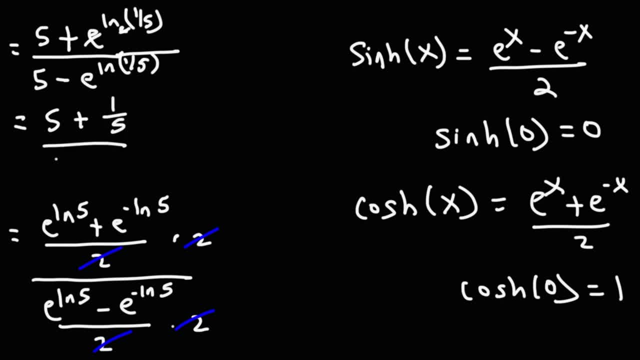 So the e's will cancel giving us 1 over 5. on the bottom, The same thing is going to happen, but it's going to be negative: 1 over 5.. So I'm going to multiply the top and the bottom fraction by 5.. 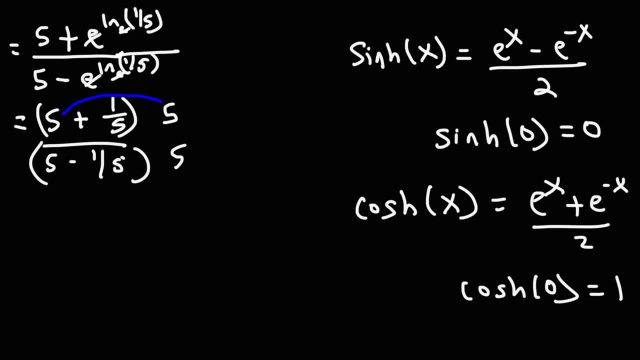 So we have 5 times. Let's do that again. 5 times 5 is It's 25.. And then 5 times 1 over 5, that's just going to be 1.. Here we have 25.. 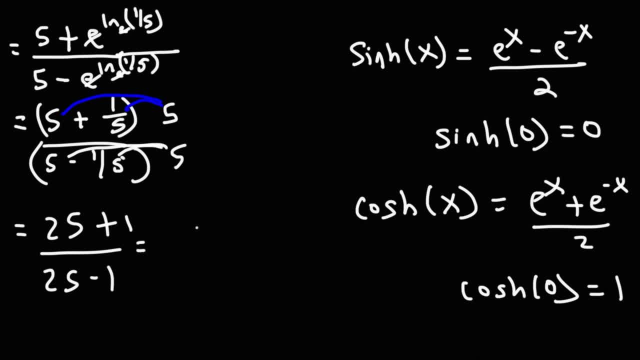 And 5 times negative. 1. fifth, that's going to be negative: 1.. 25 plus 1 is 26.. 25 minus 1 is 24.. 26 is 13 times 2.. 24 is 12 times 2.. 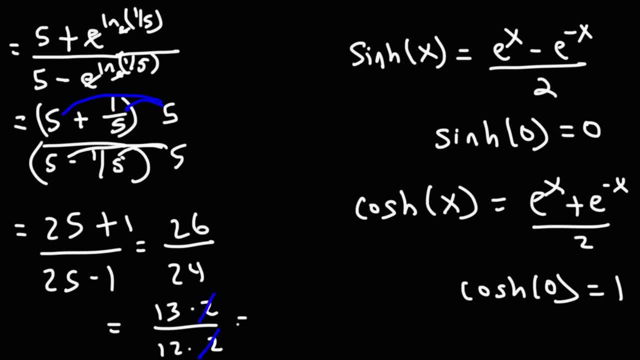 So we can cross out a 2. And this is going to be 13 over 12.. So that is the value Of cotangent natural log of 5. It's 13 over 12.. Let's try this one. What is the value of hyperbolic sine of 3?? 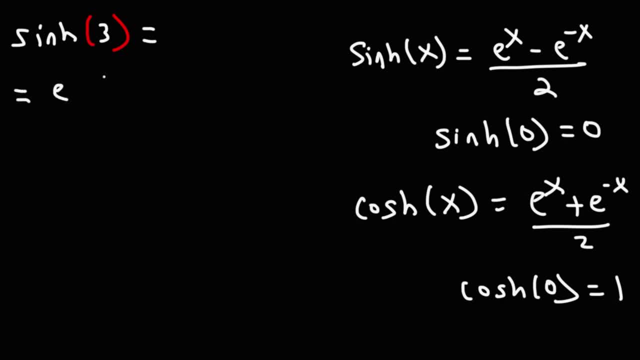 So this is going to be e to the 3 minus e to the negative 3.. So that's going to be e to the negative, 3 over 2.. So I'm going to rewrite that as 1 half e to the 3rd minus e to the negative 3.. 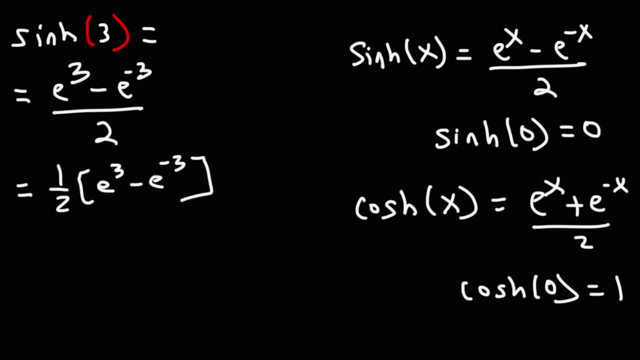 And there's really not much we can do in terms of simplifying it At this point. all we can do right now is plug this into the calculator Now. it's good to know that. e to the negative 3. This is very close. 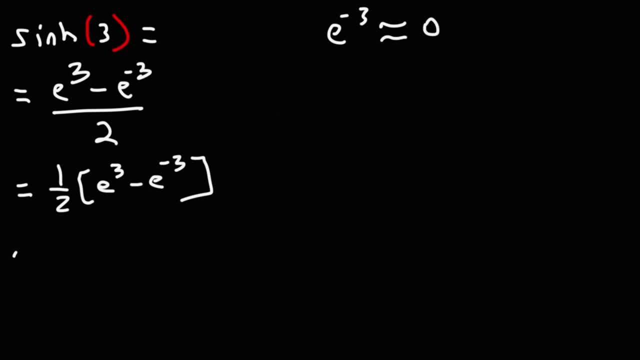 It's very close to 0. So we can approximate our answer and say it's approximately 1 half e to the 3rd. So let's go ahead and get the values for these answers. So let's start with the one on top. 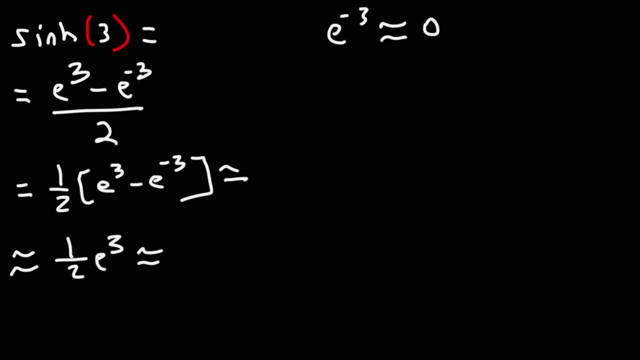 0.5 e to the 3rd, minus e to the negative 3. This is 10.0179.. As for this answer, 0.5 e to the 3rd power, it's 10.04277.. 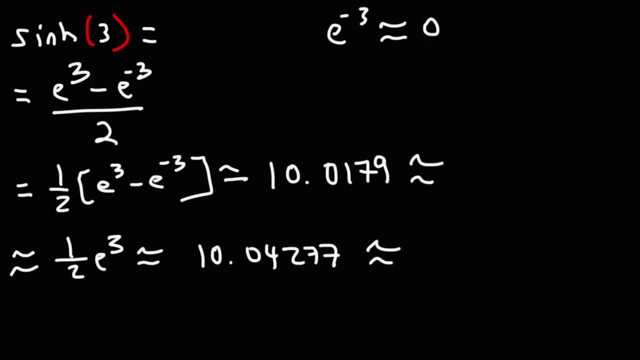 In both cases we could round the answer and say it's approximately 10.0. And we would be accurate enough. So if you want to get an approximate simplified answer, you could say it's this. If this was to the second power. 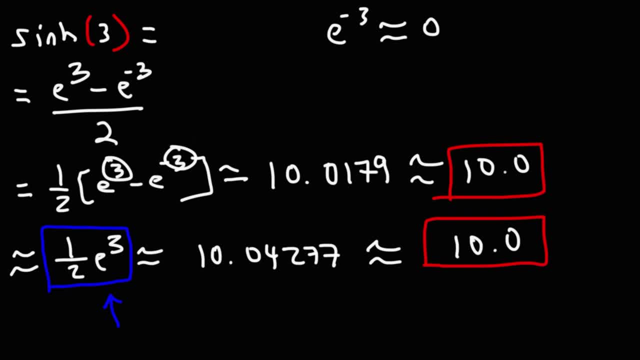 I wouldn't really get rid of this one because it might still be significant. But if it's like negative 3, negative 4, negative 5, it's going to be close enough to 0 where you can just ignore that part. 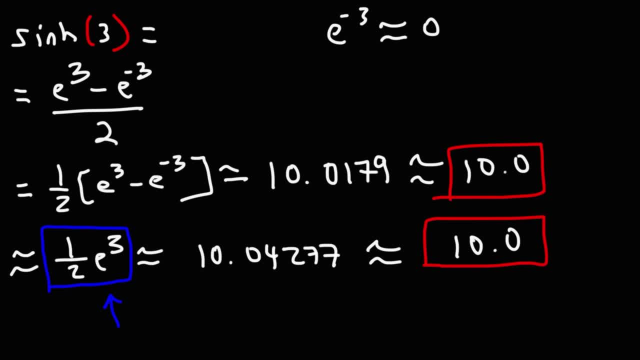 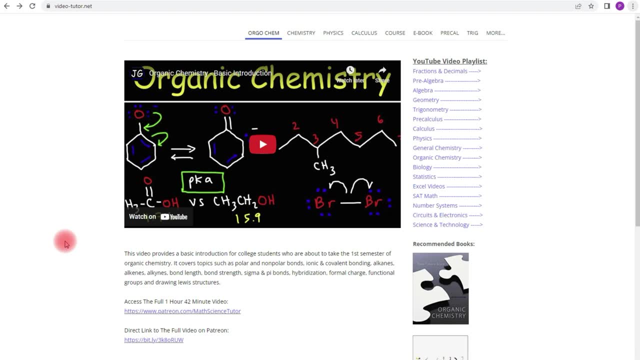 So that's basically it for this video. Now you know how to evaluate hyperbolic trick functions. Now this is for those of you who want to get access to all of my video playlists and exam review videos all in one spot. So if you go to video-2.com-